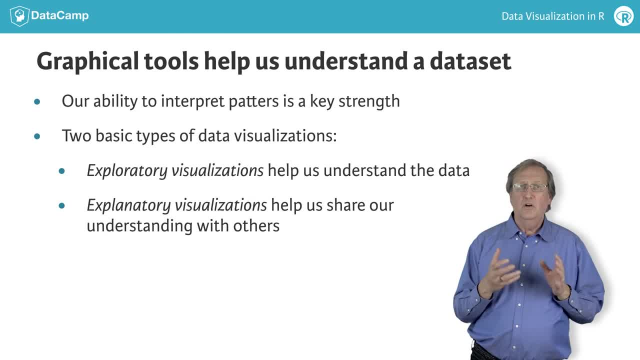 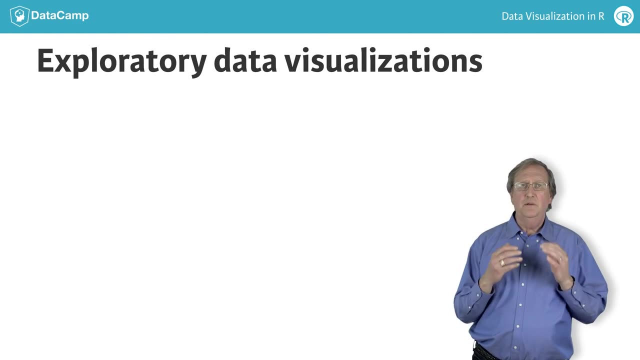 what we have found. As we will see, R provides many useful tools for creating data visualizations of both types. The key to a useful Exploratory Visualization is keeping all of the potentially relevant details. The objective is to help you see what is in the data, and the key practical question is: 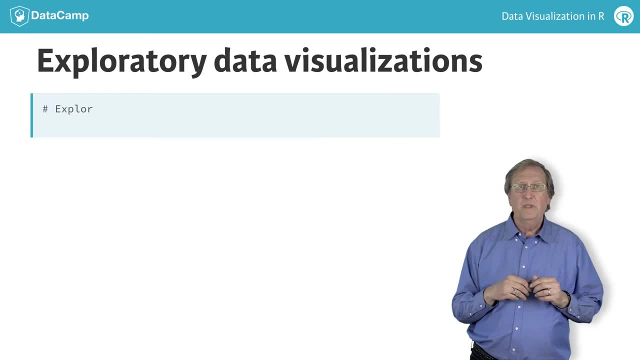 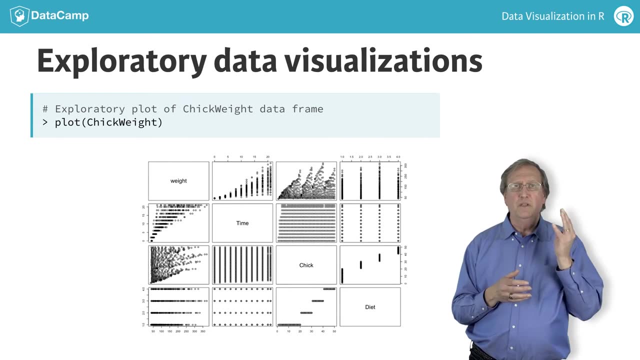 how much detail can you see and interpret? The plot array on this slide provides a representative example. It summarizes the relationships between the four variables in the Chick-Waite DataFrame in R's built-in datasets package. From these plots we can see, for example, that weight varies systematically with time. 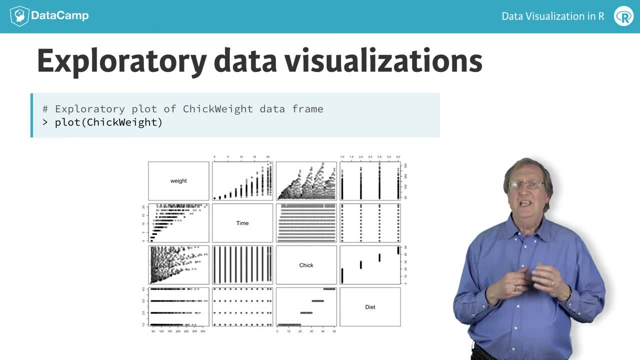 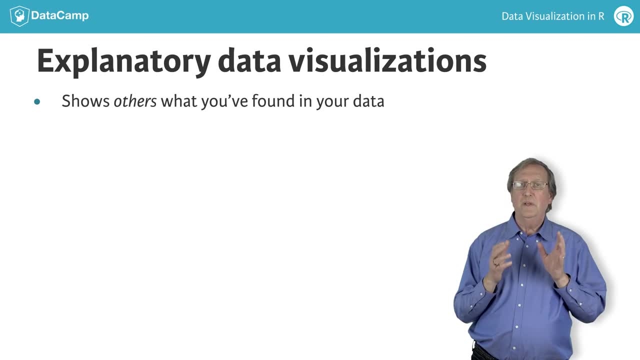 and that the chicks were assigned to four different diets. Explanatory data visualizations show others what you have found in the data. This means you must make editorial decisions. What features do you want to highlight for emphasis? What features are distracting or confusing and should be eliminated? 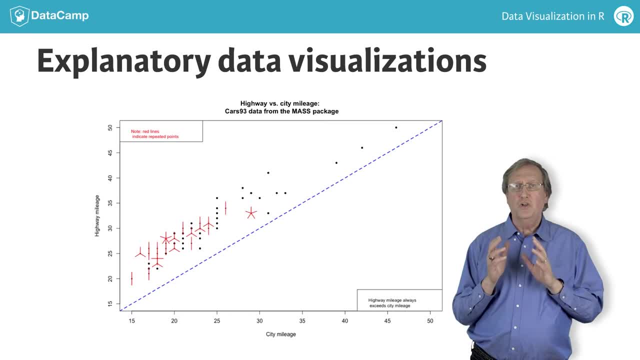 Here is an explanatory plot. The plot is constructed from the CARS93 DataFrame in the MAS package, emphasizing that highway mileage always exceeds city mileage, using techniques like reference lines and sunflower plots that you will learn about in this course. To visualize data, R supports four graphics systems. 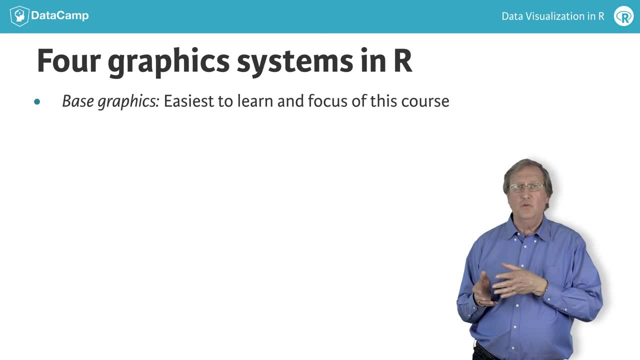 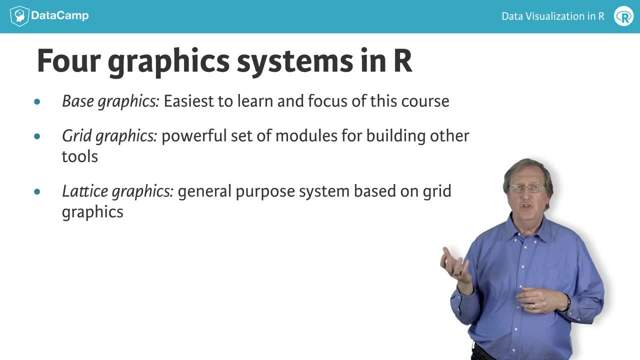 The grid graphics are the most important part of the course. This is the basis for building other tools. Lattice graphics is a general-purpose graphics system based on grid graphics, And GGBLOT2 implements the grammar of graphics in R and is also based on grid graphics. 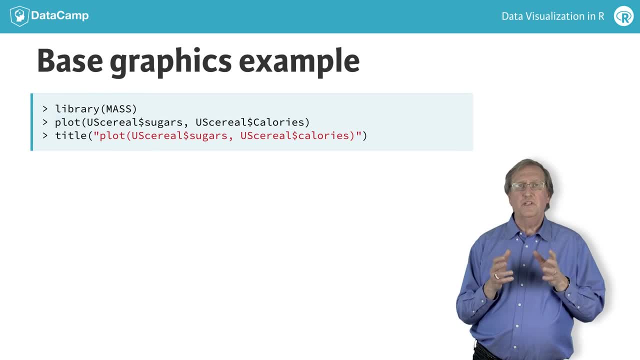 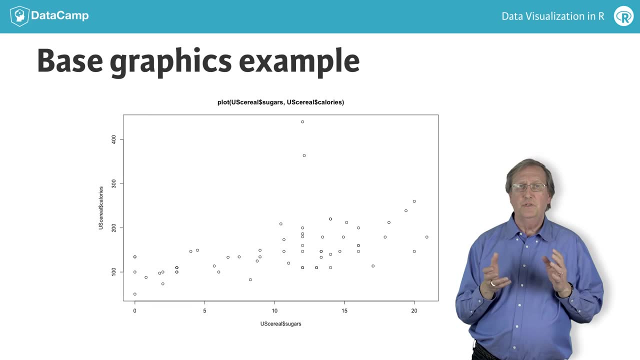 Let me give you an slide that tells us how all of this goes together. This first example uses the Base Graphics Plot function to generate simple scatterplots of calories vs sugars from the US-serial DataFrame in the MAS package. The second example uses grid graphics for developing authentication plan. however,